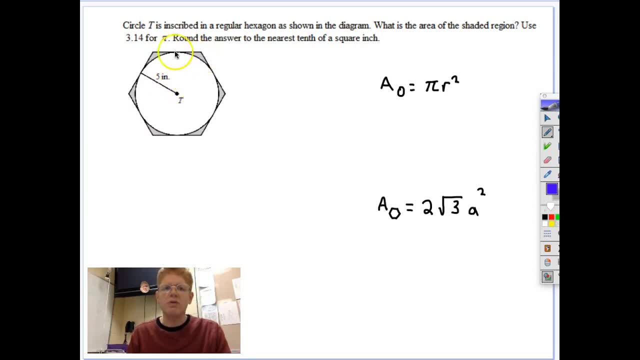 of the circle, And then we're going to subtract the two, because we want to find the area of the hexagon And then we want only the outside area. So find the area of the hexagon, find the area of the circle and then subtract the circle from the hexagon. So let's get started. The first thing, 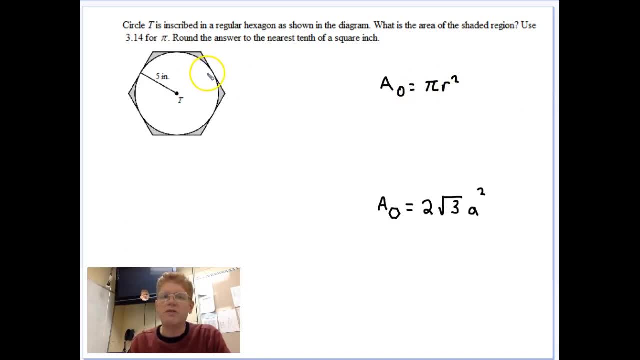 we'll do is find the area of the circle right. And we know that the area of a circle is pi r squared, because pi are not circular: Pi r squared. So we'll find that. We'll begin by marking down pi here times the radius, which is five. So we'll put that in parentheses: squared, And we know that. 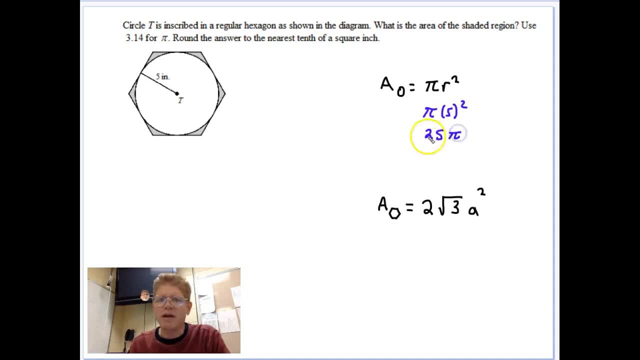 five squared is 25.. So we can write that temporarily as 25.. And then we're going to find 25 pi. That is the area of the circle, That's all the space inside of here. Then we'll find the area of the hexagon. Now, the area of the hexagon is two times the square root of three. 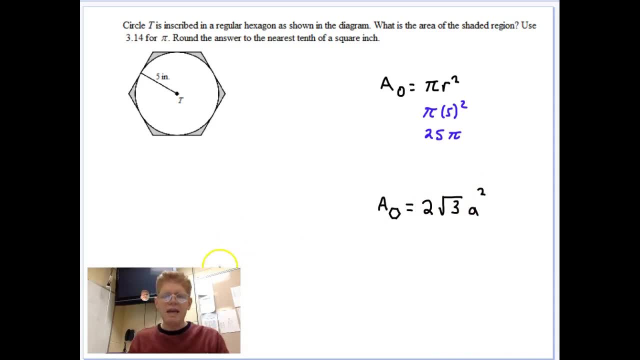 times a squared, And the a stands for the word apothem. Now, you don't have to know or remember that, but it's the word apothem And the apothem is the line that's drawn from the center to the. 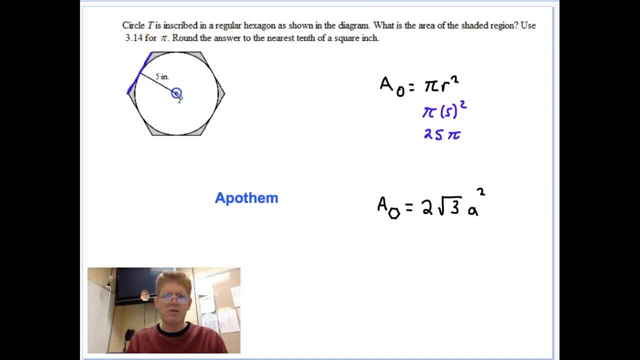 midpoint here of one of the sides, from the center of the hexagon to the midpoint of its sides, called the apothem, And we square that. So in our case it turns out that that is also the radius of our circle. So what we are going to do is, in place of a, we're going to plug in the 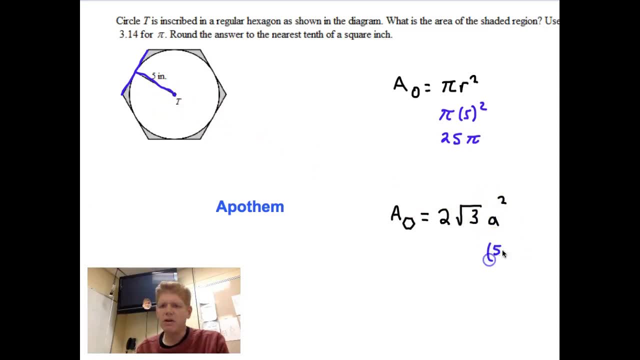 value of our radius up here: five inches, So five. we're going to square that And we're going to multiply that by two times the square root of three. Now, five squared is 25.. And we're going to multiply that by two times the square root of three. But because of the commutative and 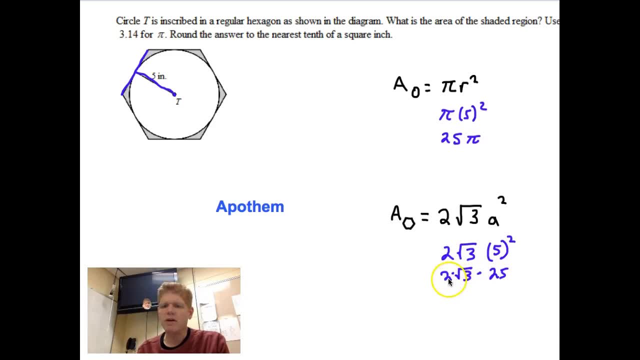 associative properties. we can group these guys, rearrange them up, and we're going to be able to do them, however we need to, because it's multiplication, And we'll multiply two times 25, which gives us 50.. 50 times square root of three, And that is the best way to write our 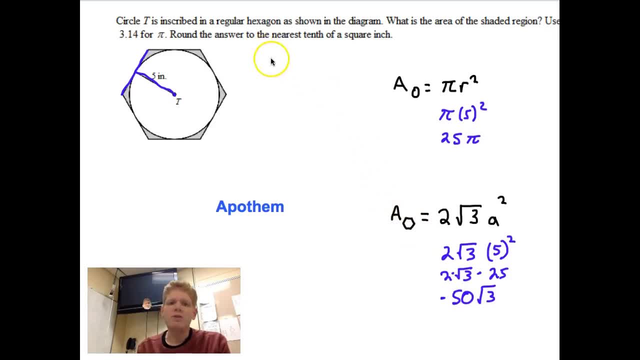 area of our hexagon for now, And what we need to do is then subtract those two values. So- and that's not a negative, by the way, that's a star- So we'll star both of those And what we'll do is we'll take 50 square root of three And from that we will subtract 25.